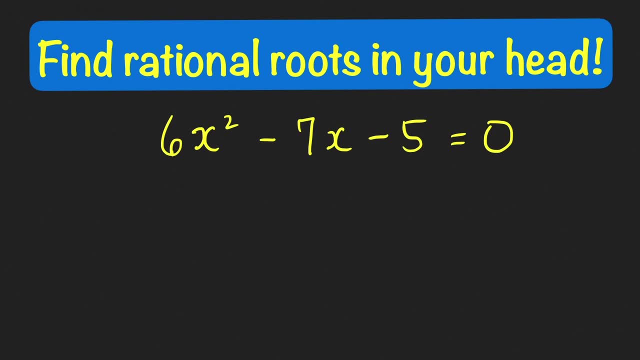 of this equation in my mind. then I'll think of factors of the product of 6 and negative 5, which is negative 30. Whose sum is the negative of this, which is equal to 7?? So what are the factors of negative 30? Whose sum is positive 7?? So those are positive 10 and negative 3.. So in this case, 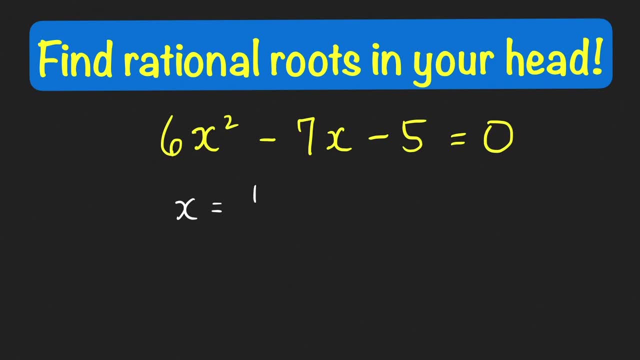 I know already, The roots are 10 over 6 and then negative 3 over 6.. So where did I get the 6 here? This 6 here is just the coefficient of your x squared term, And these solutions or roots can be simplified to 5. 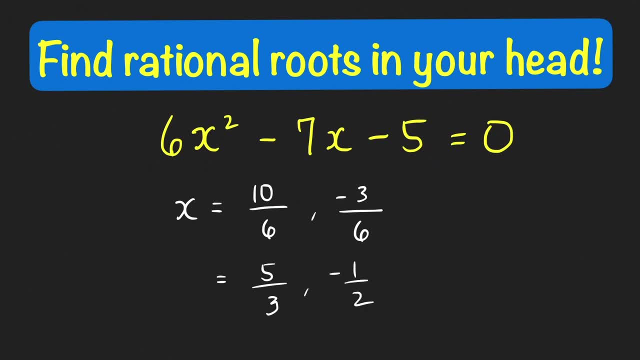 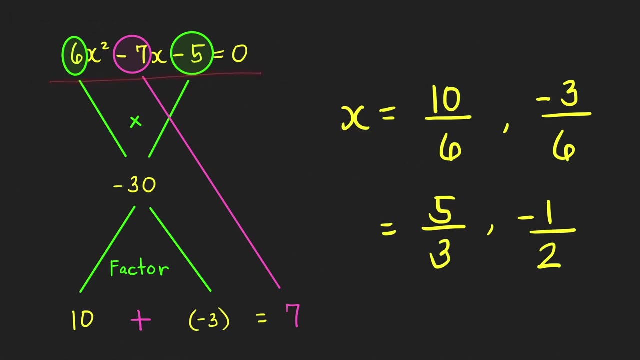 over 3 and negative 1 half, And you can check that these are indeed the solutions of this equation. Let me explain the process step by step. So this is our quadratic equation. So it's in the form: ax squared plus bx plus c, equal to 0.. So the first step is to multiply the a and c. So that is. 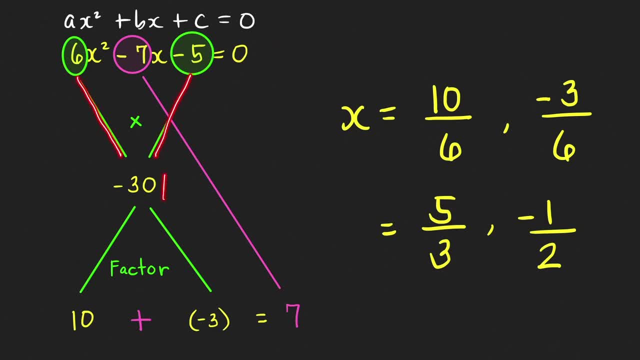 we take the product of 6 and negative 5 and we'll get negative 30. So this is the product of a and c, And now you think of factors of this negative 30. Whose sum is the negative of this? So you take the negative of this one and that is equal to 7.. So this is just the negative of the. 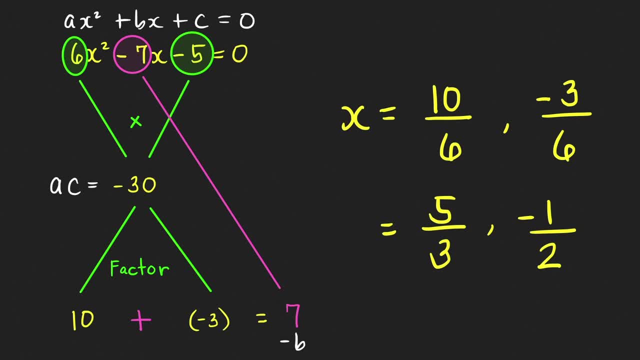 coefficient of x. So what are the factors of negative 30?? Whose sum is 7?? They are 10 and negative 3.. And after finding this, I'll take the product of 6 and negative 3 over 6.. So this is: 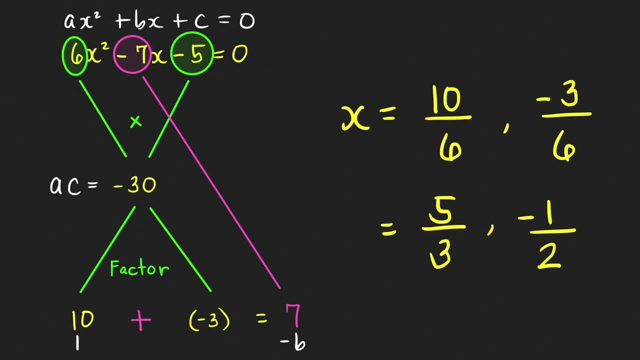 appropriate factors, So we may label them as m and capital N. You can already determine the solutions of the quadratic equation, and they are: what x equals m over a, where a is the coefficient of your x squared, and then n over a. So here we have 10 over 6 and negative 3 over 6, which can 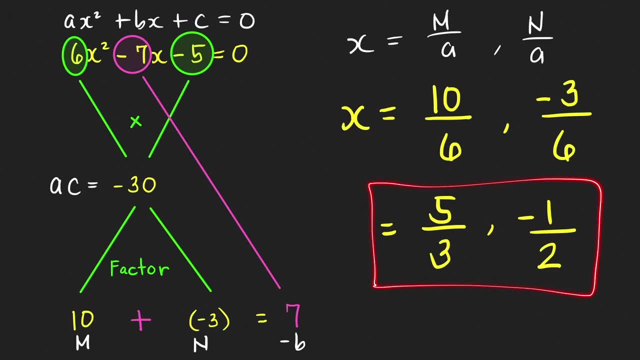 be simplified to 5 over 3 and negative 1.. So to understand why these two numbers here are solutions of this equation. here you may watch my other video, which talks about factoring of a trinomial of the form ax squared plus bx plus c. The link to this video is given in the information section in the upper right. 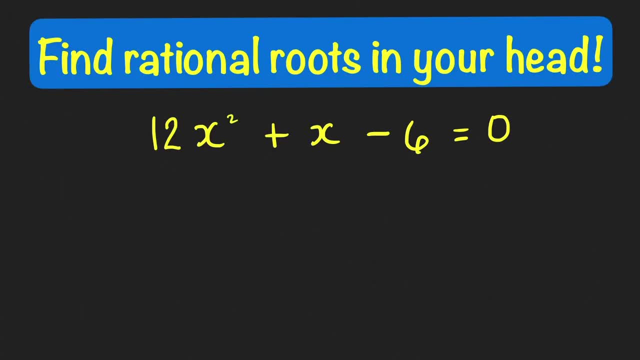 corner. Let's give one more example. So let's say we want to find the roots of this quadratic equation here. So we're going to find the roots of this quadratic equation here. So we're going to 12x squared plus x minus 6 equal to 0. So how do we find the roots mentally? So again we think of: 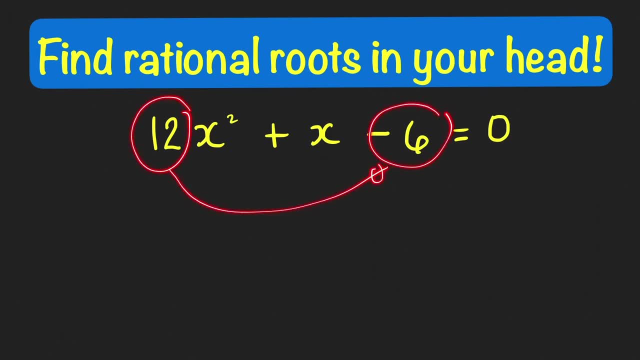 factors of the product of 12 and negative 6.. So that is negative 72.. Whose sum is the negative of the coefficient of x? So whose sum is negative 1?? So what are the factors of negative 72?? Whose sum is negative 1?? 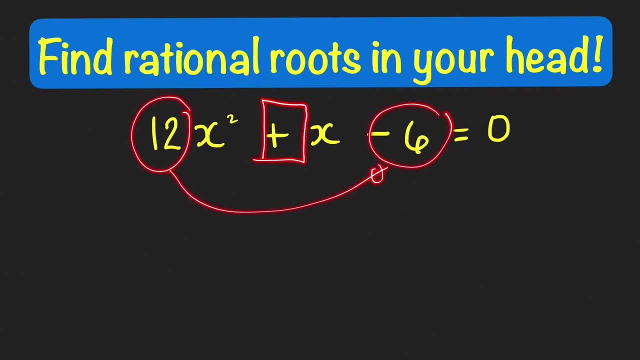 And we can easily determine those factors. They are negative 9 and 8.. And therefore the solutions of this quadratic equation is negative 9 over the coefficient of x squared, which is equal to 12, and then positive 8 over the coefficient of x squared over 12.. And we can simplify this to: 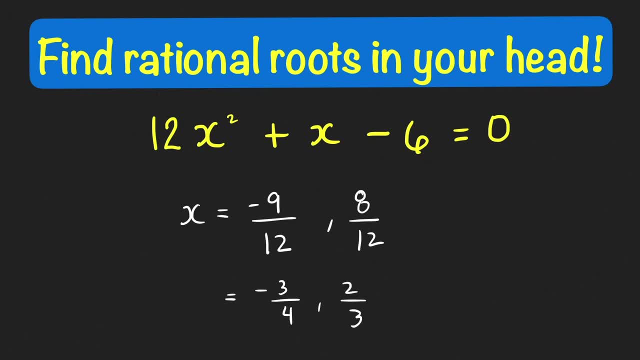 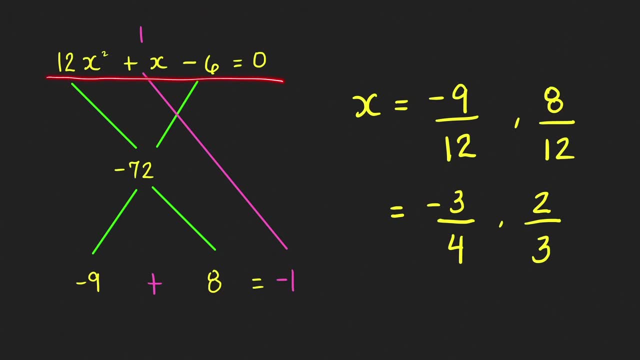 negative, 3 fourths and 2 thirds. So again, let me show you how to find the roots of this quadratic equation. So let's show the step-by-step process. So we're given this equation here. First step is to multiply this a and c And we'll get here negative 72.. And then after that we think of: 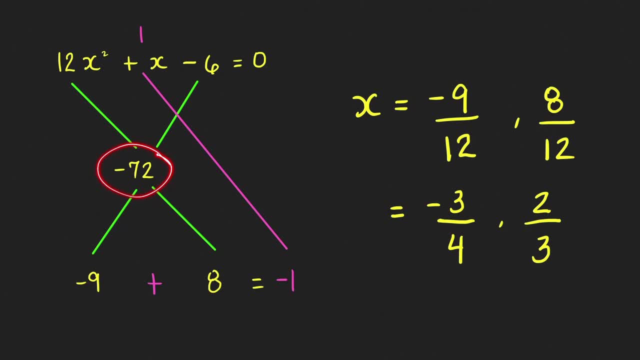 factors of this product, whose sum is the negative of the coefficient of x And the negative of the coefficient of x. this is your negative b, That is equal to negative 1.. And after finding these factors, here, m and n, we can already find the solutions, which are m over.